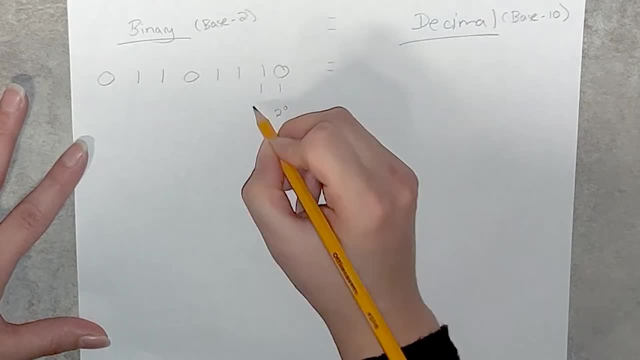 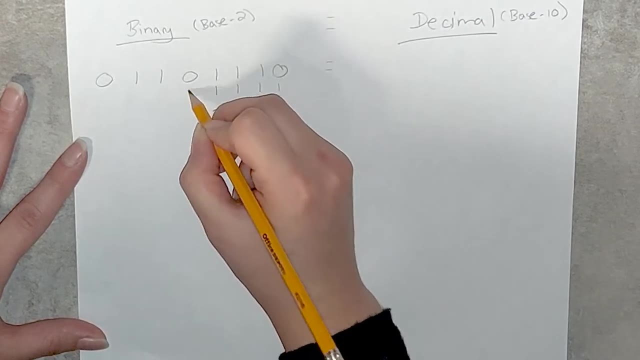 So this one is 2 to the 0, this one's 2 to the power of 1, this one's 2 squared, 2 to the power of 3, 2 to the power of 4.. This is why I spaced them out, so I had room to write this. 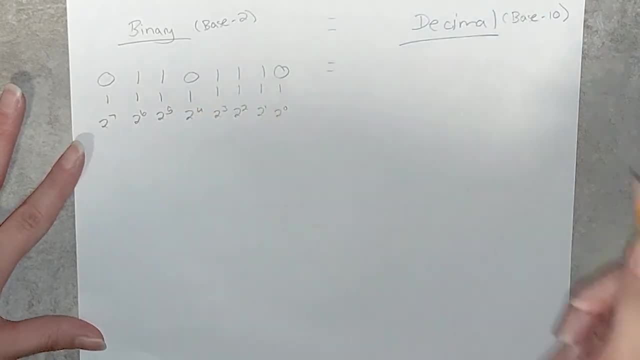 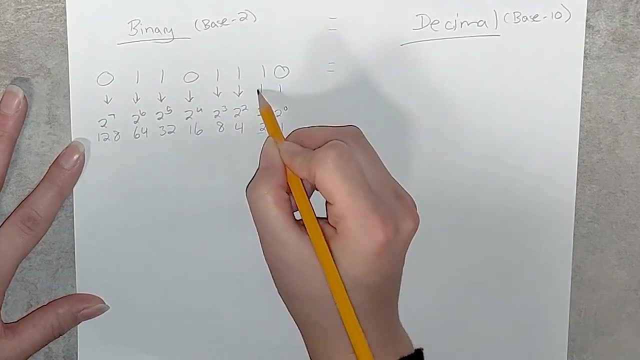 2 to the power of 6, and 2 to the power of 7,, which is equal to 1,, 2,, 4,, 8,, 16,, 32,, 64, and 128.. I should have made, I should make this a little more clear so that doesn't look like ones. 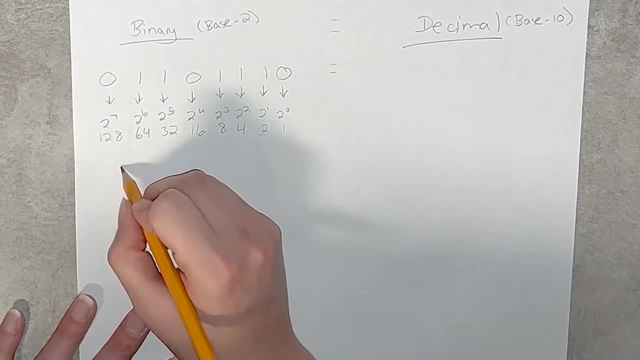 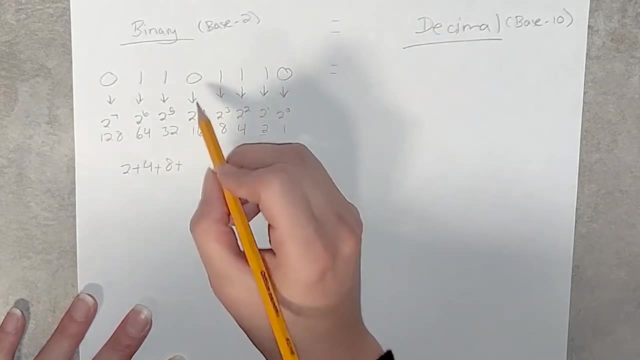 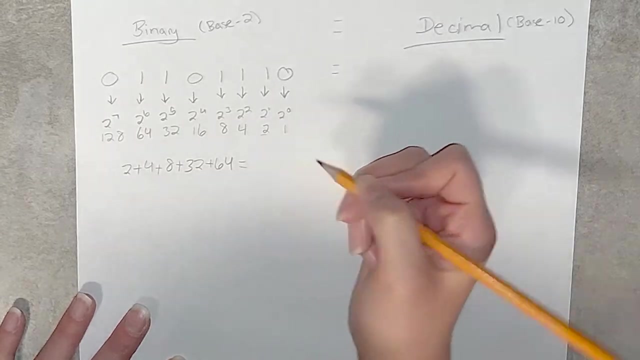 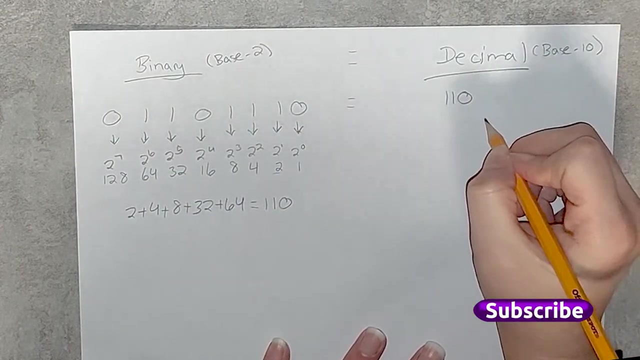 So we add the place value, So we have 2.. We have 4.. We have 8.. Nothing in the 16th place, Something in the 32 place, Something in the 64 place- 110.. So that is our decimal value. 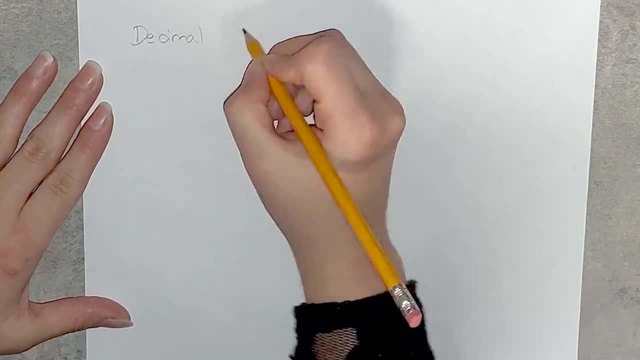 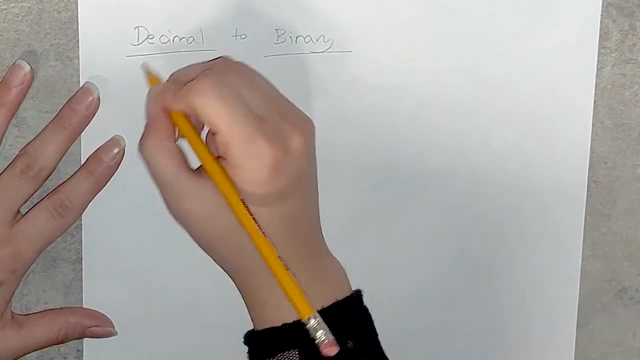 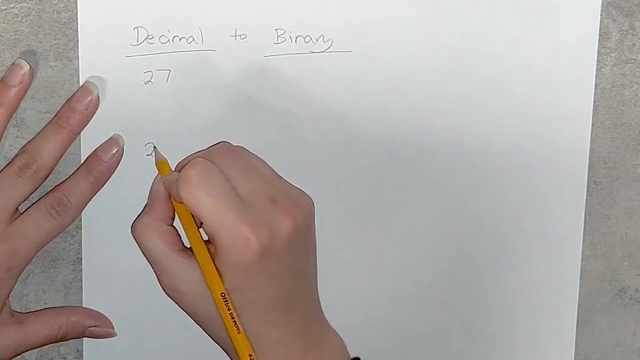 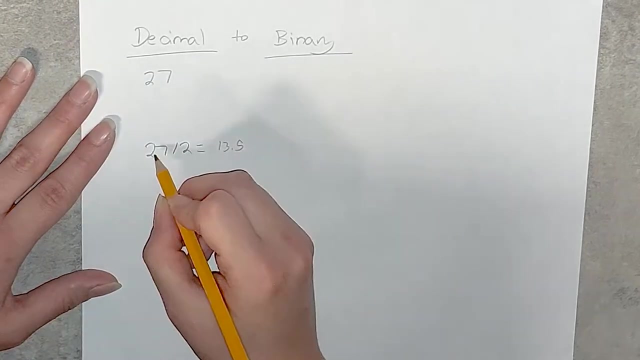 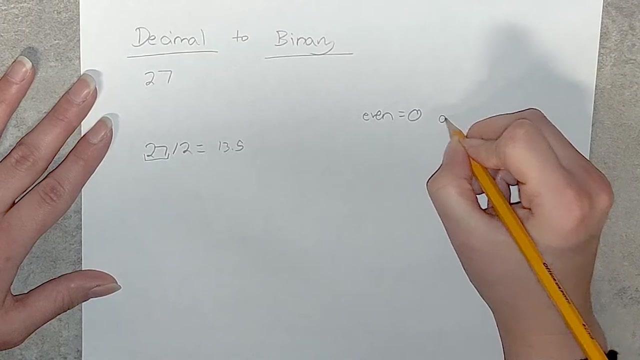 Now, if you want to go decimal to binary, You just have to divide by 2 a lot, so it's 27,. so take your original number and divide it by 2, so it's 13.5, right, Your rightmost bit depends on this number, right here. so if it's even, we're going to write a 0,, if it's odd, we're going to write a 1.. 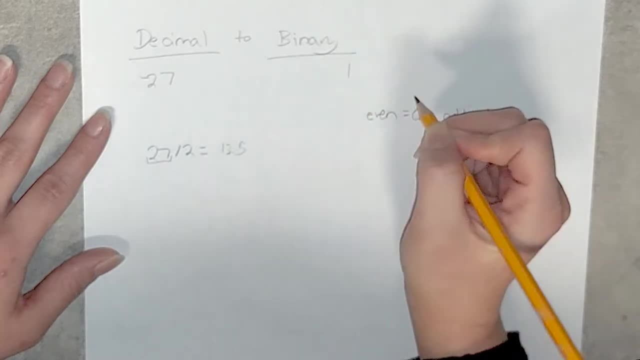 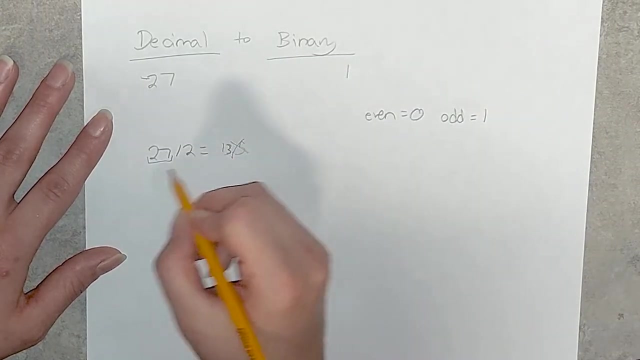 So this is odd. so our rightmost bit is 1.. So this is odd, so our rightmost bit is 1.. And as for this remainder, let's truncate it. So the next number is 13,, not 13.5,, just 13.. 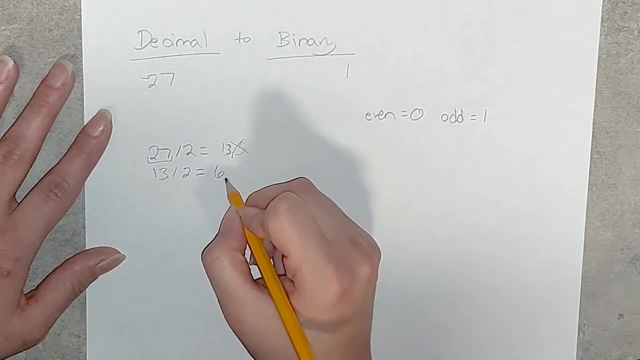 13 divided by 2 is 6.5,, but we're just going to write 6.. And because 13 is odd, it means that our next number is 1.. And 6 is even so. our next number is 0.. 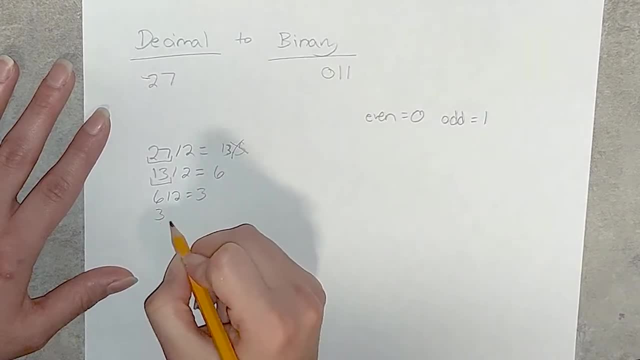 6 divided by 2 is 3.. 3 is odd, so a 1. That divided by 2 is 1.5, or 1. 1 is odd, so another 1. Divided by 2 equals 0..